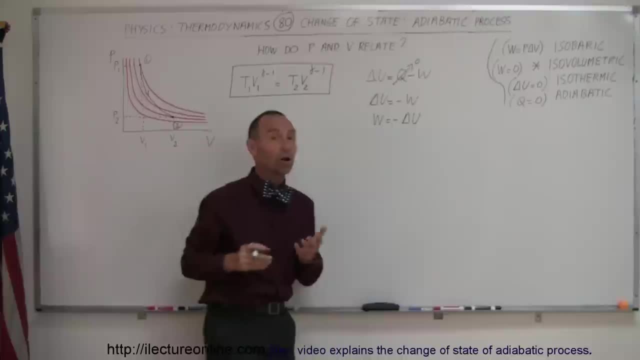 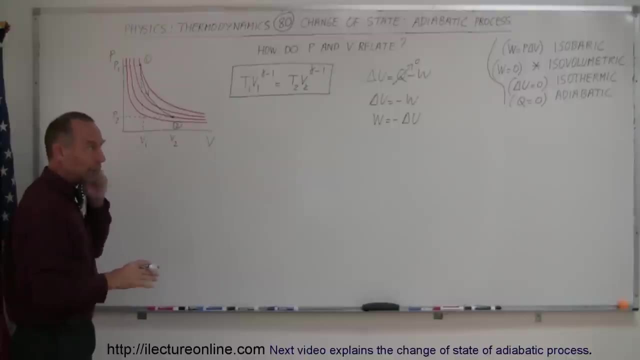 equal to minus the change in internal energy. In other words, all of the energy that is going to that it needs to do work came from within the energy of the gas. Now, by using that in the first law of thermodynamics and the gas equation, PV equals nRT, and going through some 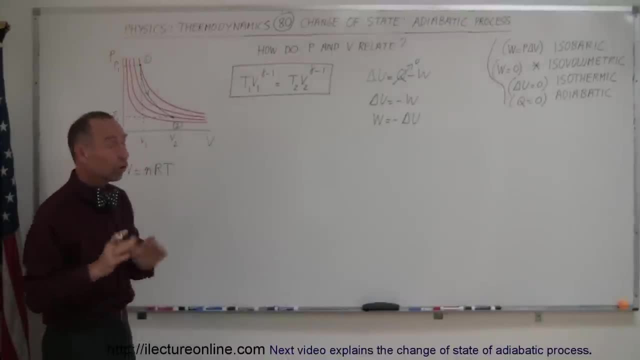 lengthy derivation, we're able to come up with this relationship, But we should also be able to come up with the relationship between pressure and volume in an adiabatic process, And so what we're going to do now is utilize this equation along with this, And what we're going 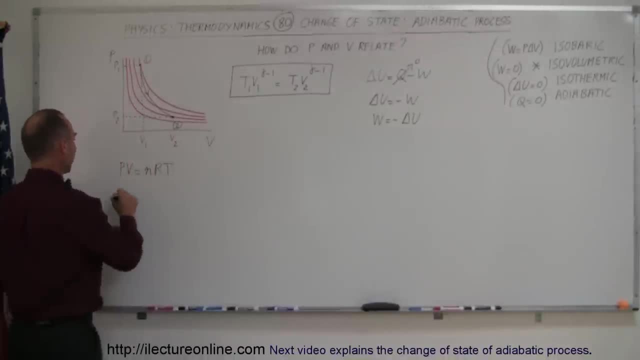 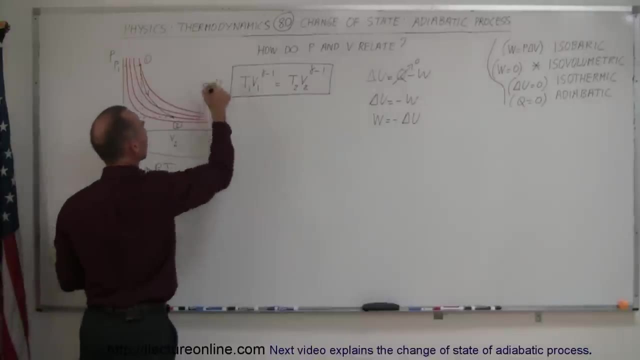 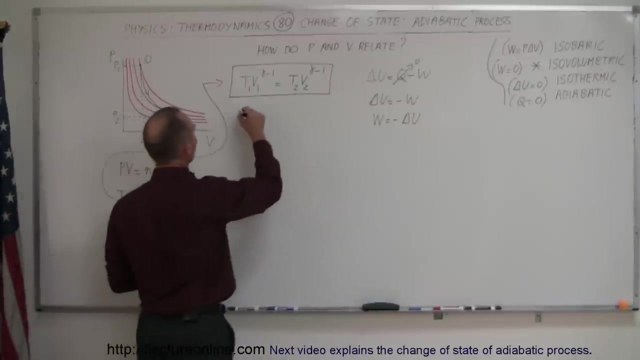 to do here is: we're going to solve this equation for T, So we say that T is equal to PV divided by nR and plug that into our equation over here, And when we do that, so instead of course T1, we're going to write P1V1 over nR, So that is P1V1 over nR times V1 to the gamma minus. 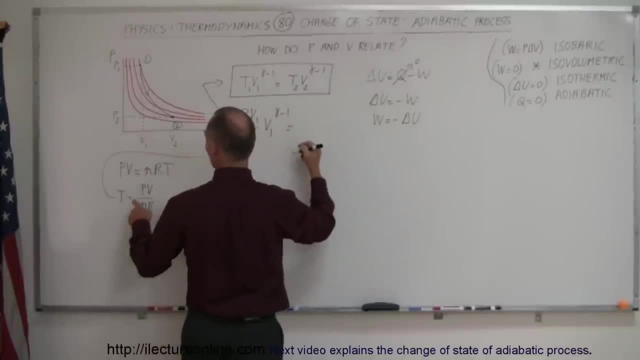 1.. And then instead of T2 we're going to write P2V2.. So we multiply P2 here P1.E2.E2,. you can divide P2 by an finding: 4, 1 over nr which. 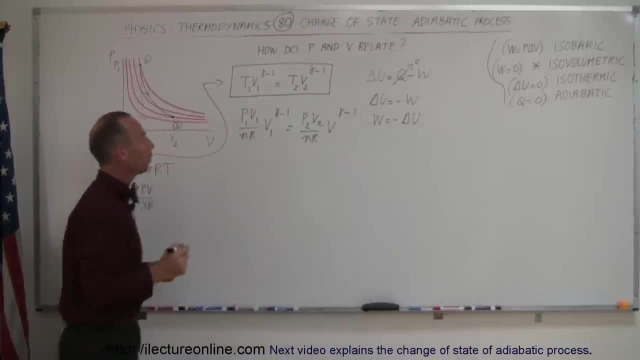 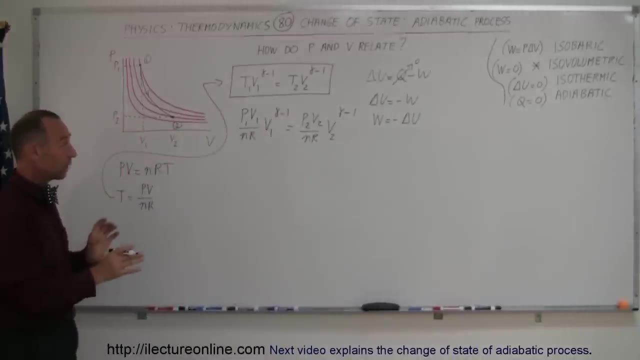 is going to be p2, So P2V2, p2 over nR times volume to the gamma minus 1, um, and of course I do want a 2. there can't forget the 2.. Alright, now, when we look at that one, on both sides of the equation we have divide by nR. 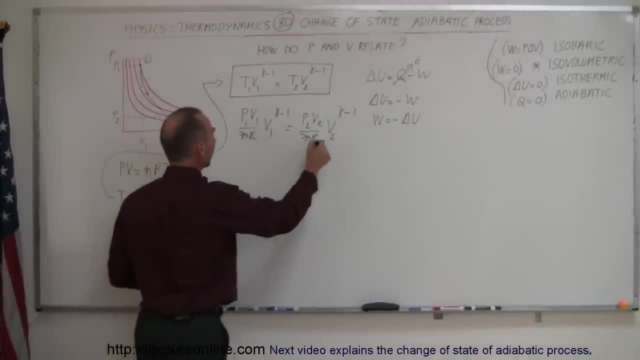 and n and r are constants, So we can go ahead and cancel that out. So the equation now becomes: P1V1 times V1 to the gamma minus 1, equals P2V2 times V2 to the gamma minus 1, all right. 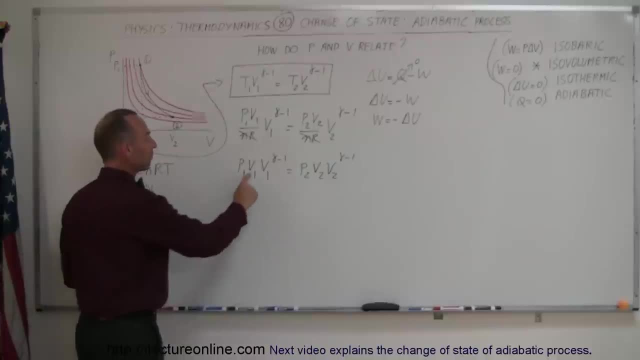 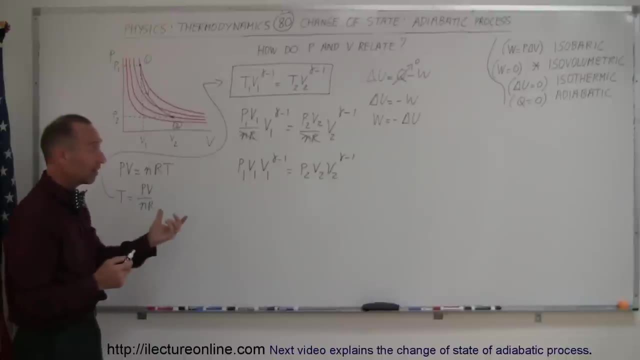 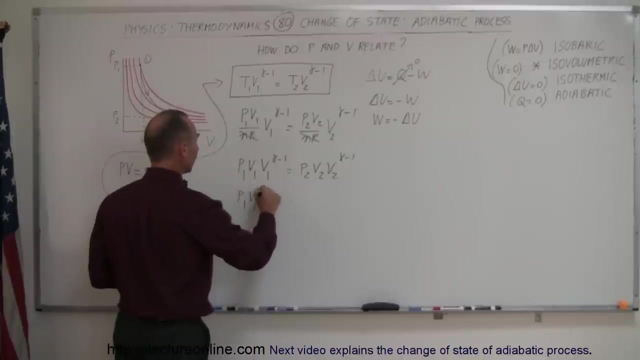 minus 1. so here we have an interesting situation. we have v1 times v1 to the gamma minus 1. so here we're multiplying two things together and the bases are the same. that means we can add the exponents. of course, the exponents to this one is 1, so this becomes p1, v1 to the gamma minus 1. 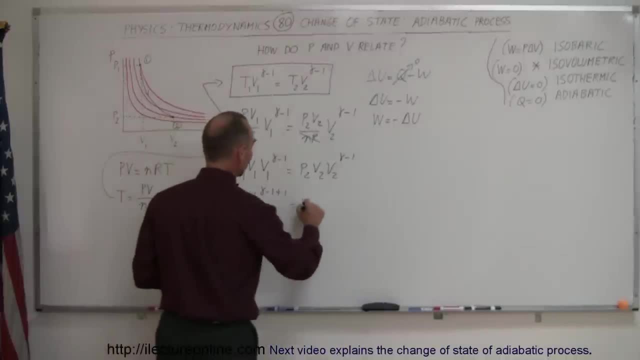 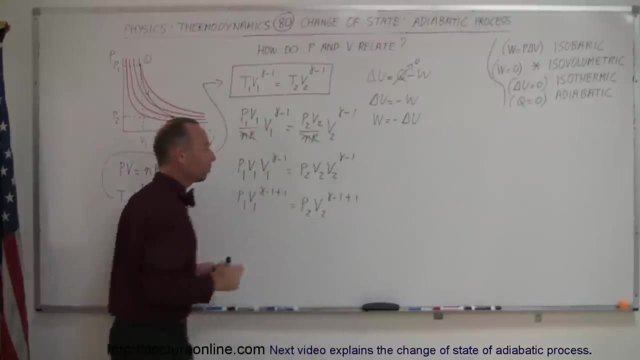 plus 1- that's the exponent from this v1- equals p2 v2 to the gamma. minus 1 plus 1 again, that's plus 1 from this v2, right there. notice then that the ones cancel out and we end up with p1 v1 to. 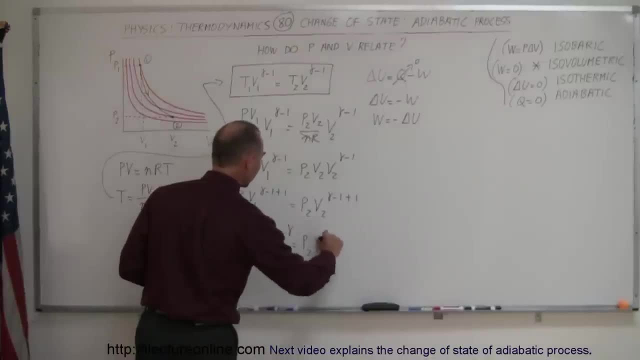 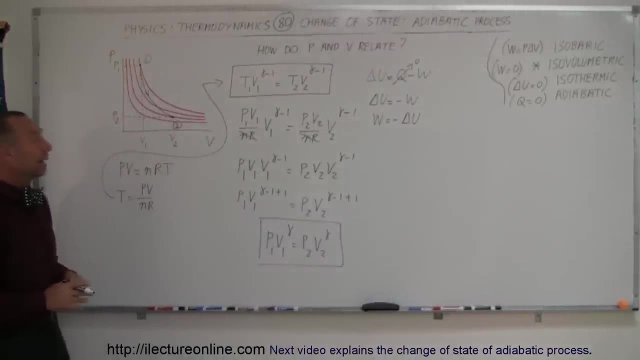 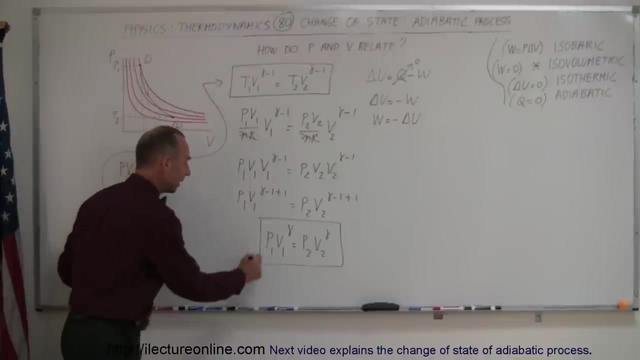 the gamma equals p2, v2 to the gamma, and here we now have a new relationship between two of the state variables for the gas in the nativatic process. so here we can relate t1, t and v, and here we can relate p and v. and these two equations are really helpful and you'll see in some in the 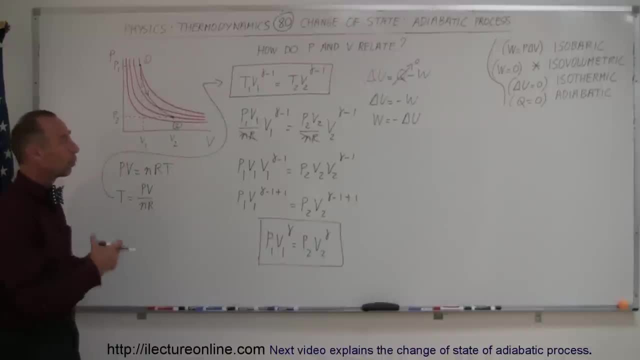 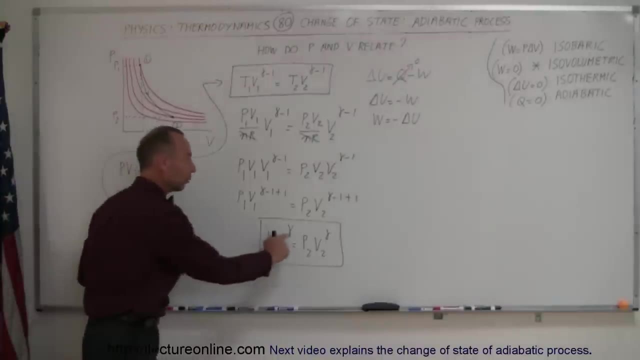 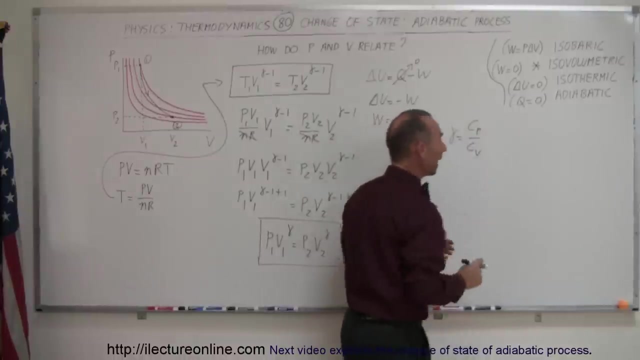 following video how to use those equations to come up with the work done and the change in the internal energy of a gas in an adiabatic process. again, if you don't remember what the gamma stands for, remember that gamma is equal to the ratio of c sub p divided by c sub v, and those values are: 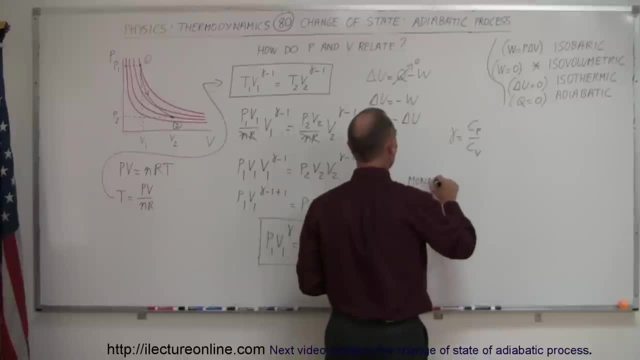 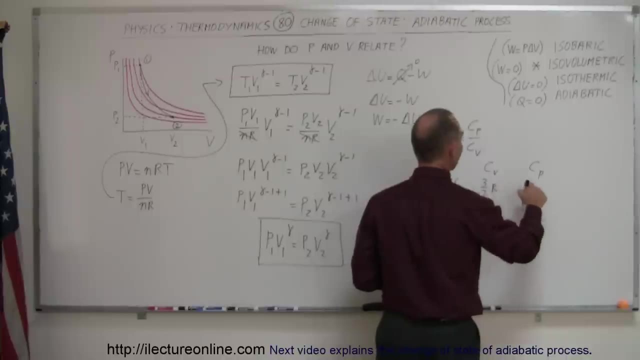 equal to depending upon what gas you're talking about. if we have a monatomic gas and we have c sub v and have c sub p, for monatomic gas, c sub v is 3 over 2 r and c sub p is 4 and c sub p is 6 and c sub p is 6 and c sub p is 7. 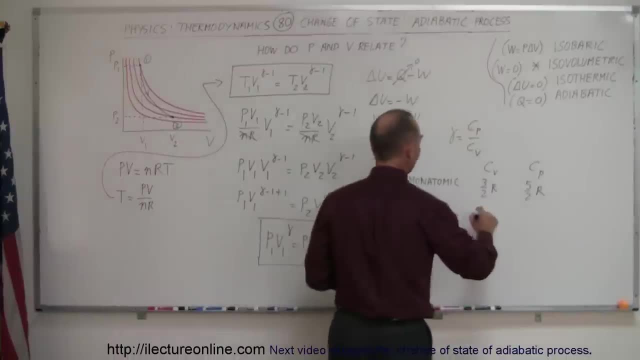 5 over 2R. For a diatomic gas, C sub V is 5 over 2R and C sub P is 7 over 2R, And for a triatomic gas, C sub V is 7 over 2R and C sub P is 9 over 2R. Now again, these are not exact values. They. 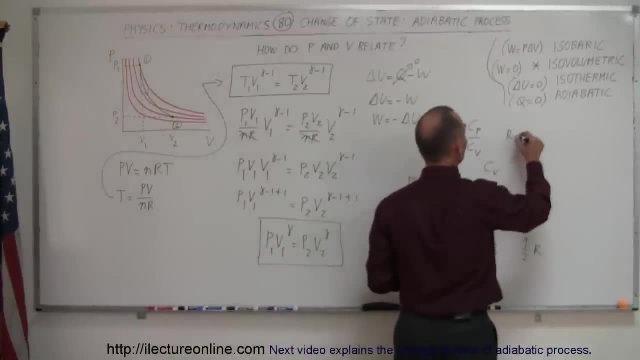 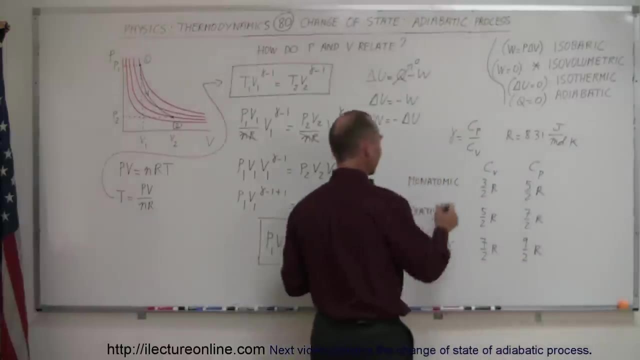 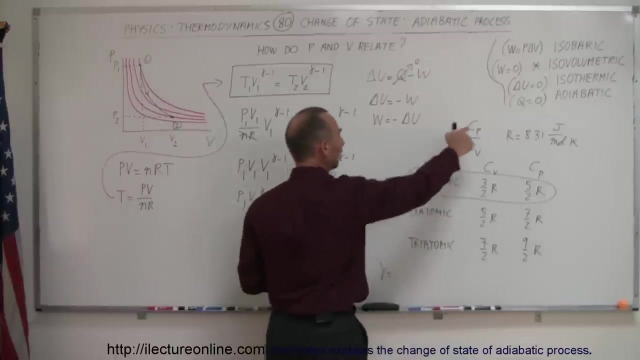 are approximate values And also, if you don't remember, R is equal to 8.31 joules per mole times Kelvin And, for example, if we take a monatomic gas as an example, we want to calculate the gamma. for a monatomic gas. That would be. gamma is equal to C sub P divided by C sub V. 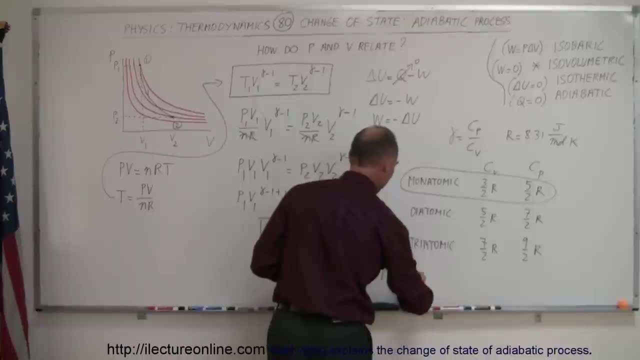 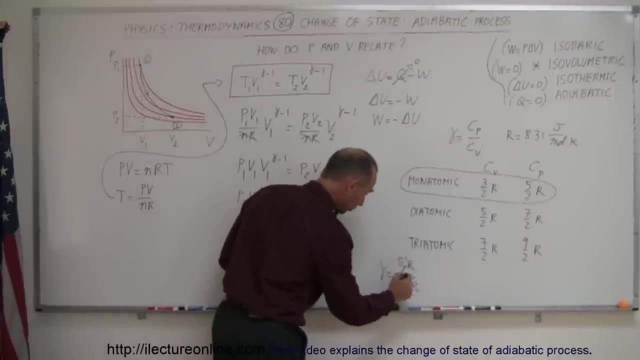 The C sub P would be 5 over 2R. The C sub V would be 3 over 2R. Notice then that the R's will cancel out, The divided by 2's will cancel out. So we end up with this equal to 5 over 3,, which is equal to. 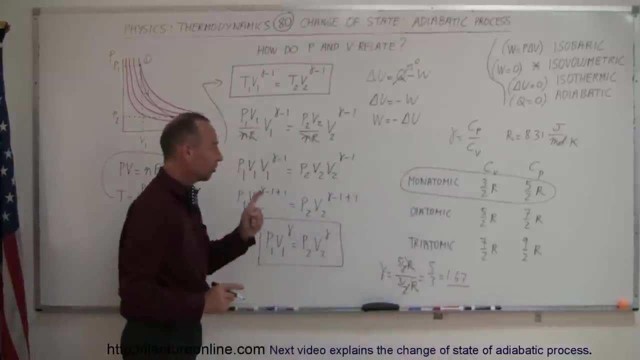 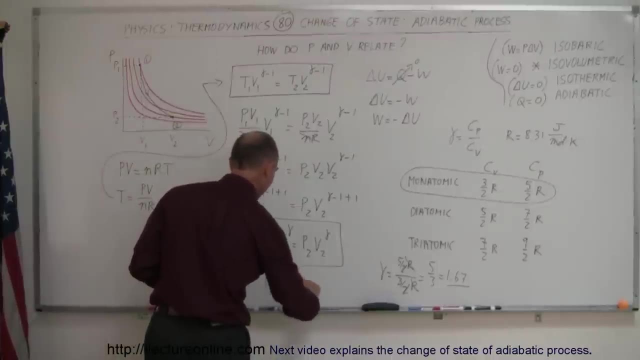 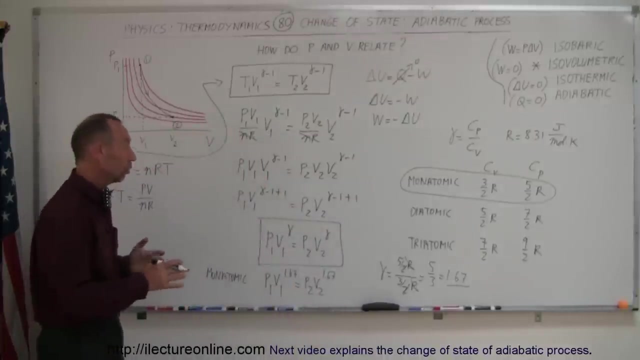 1.67.. So you can see, then, for a monatomic gas, this equation becomes: P1 V1 to the 1.67, equals P2 V2 to the 1.67.. And so that's how this equation is adapted to the gas, depending upon if it's a monatomic gas or a. 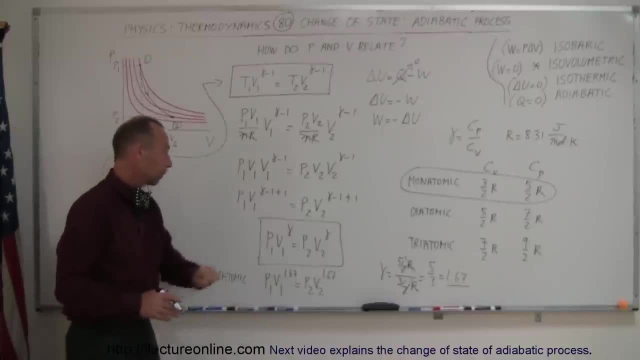 diatomic gas or a triatomic gas. For a diatomic gas, this would become 1.4.. For a triatomic gas, this would become 9 over 7, which I'd have to calculate that out. Matter of fact. I have a.